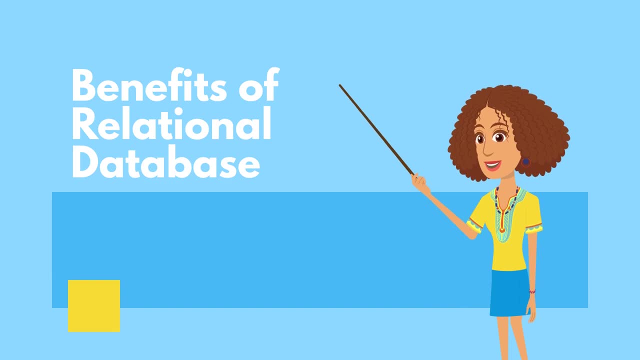 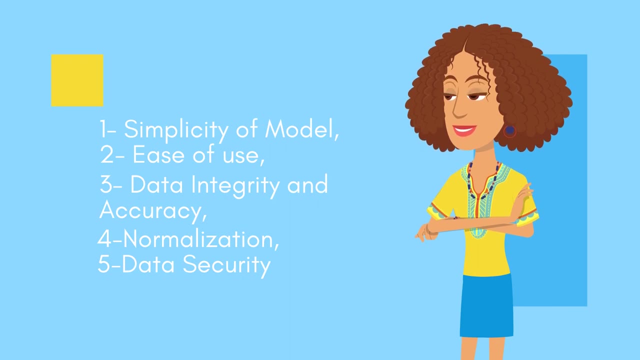 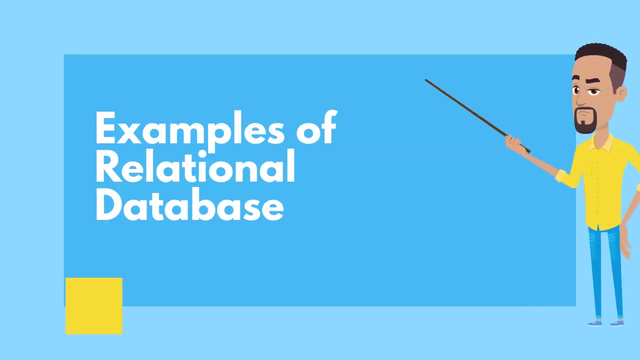 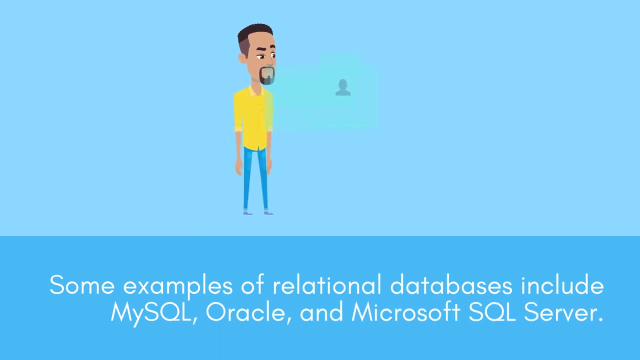 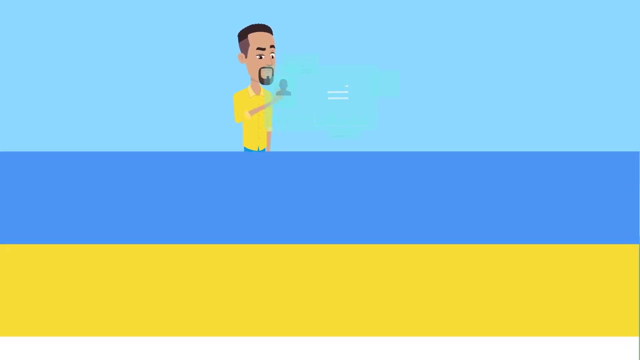 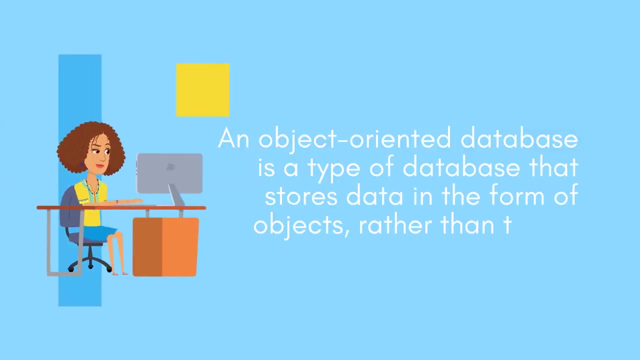 Benefits of relational database: 1. Simplicity of model, 2. Ease of use, 3. Data integrity and accuracy, 4. Normalization, 5. Data security. Examples of relational database. Examples of relational databasez include MySQL, Oracle and Microsoft SQL Server. 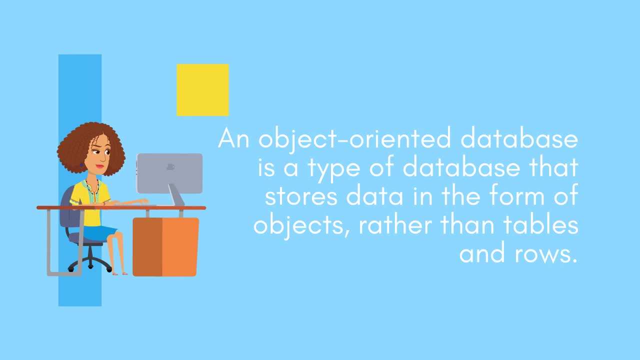 Some examples of relational databases include MySQL, Oracle and Microsoft SQL electrical servers. What is an object oriented database? An object-oriented database is a type of database that stores data in the form of objects rather than tables and rows. What is an object oriented database? An object-oriented database is a type of database that stores data in sex of groups or in the form of groups rather than tables and rows. These objects are organized and stored in order to exist. in a random, array-based data source, It means an object yearn in such a database would naturally facilitate the public to organize. 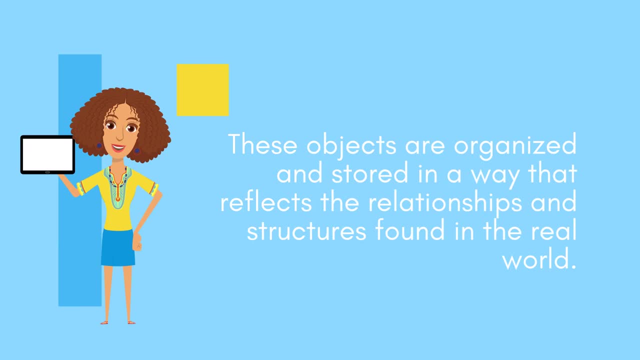 different kind of output and type And it means a very fast process of 73 percent data, traditional data, in such a JPEG implement. There are three dimensions in terms of matter, especially the classe, object, nature and data technology stored in a way that reflects the relationships and structures found in the real world. 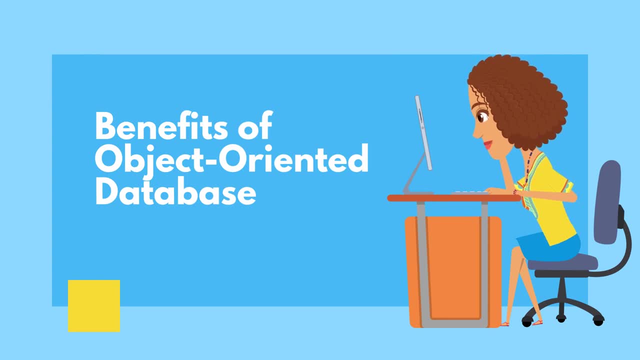 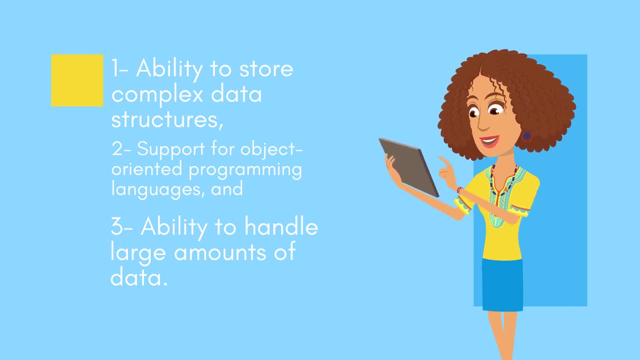 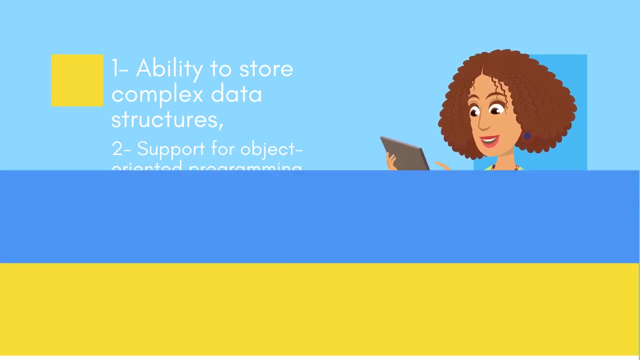 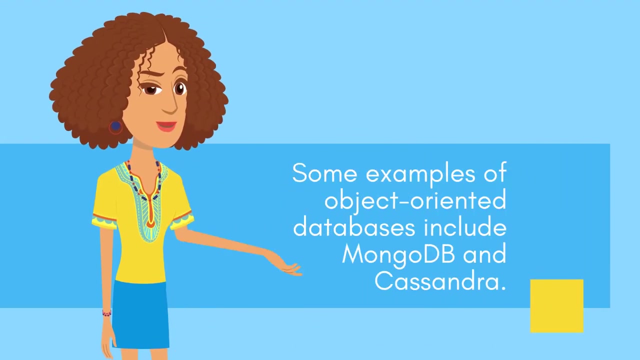 Benefits of Object-Oriented Database: 1. Ability to store complex data structures. 2. Support for object-oriented programming languages. 3. Ability to handle large amounts of data. Examples of Object-Oriented Database. Some examples of Object-Oriented Databases include MongoDB and Cassandra. 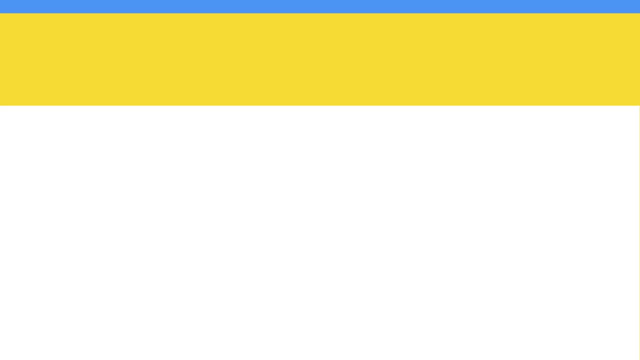 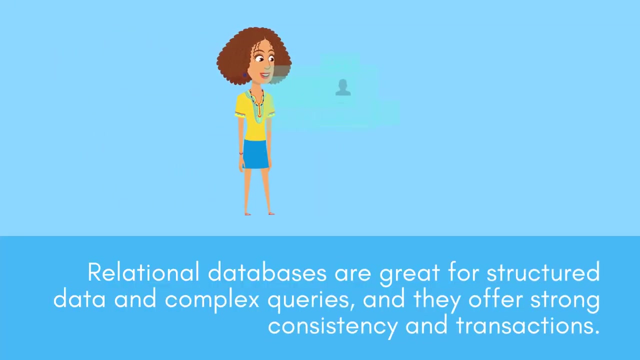 So which type of database is right for you? It really depends on the needs of your project. Relational databases are great for structured data and complex queries, and they offer strong consistency and transactions. Object-Oriented Databases. Object-Oriented Databases. 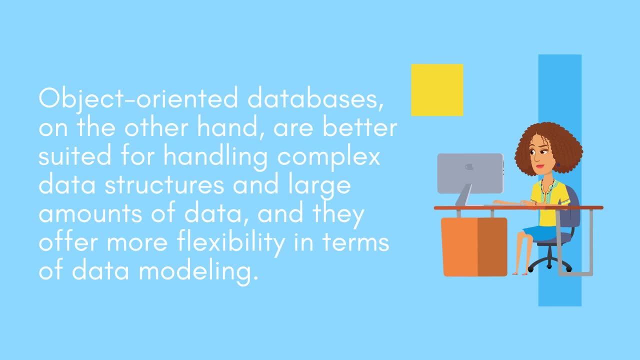 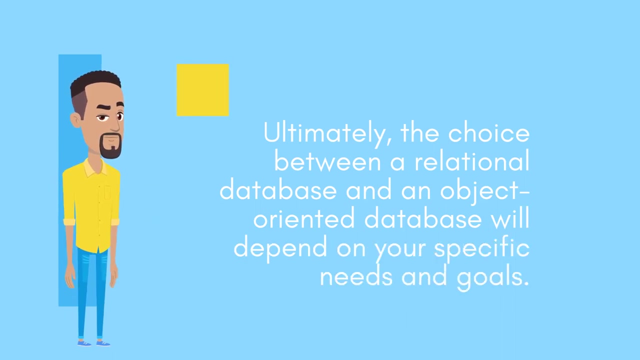 Object-Oriented Databases, on the other hand, are better suited for handling complex data structures and large amounts of data, and they offer more flexibility in terms of data modeling. Ultimately, the choice between a relational database and an object-oriented database will depend on your specific needs and goals.